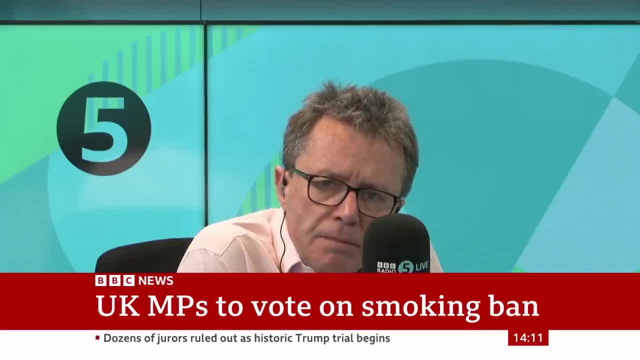 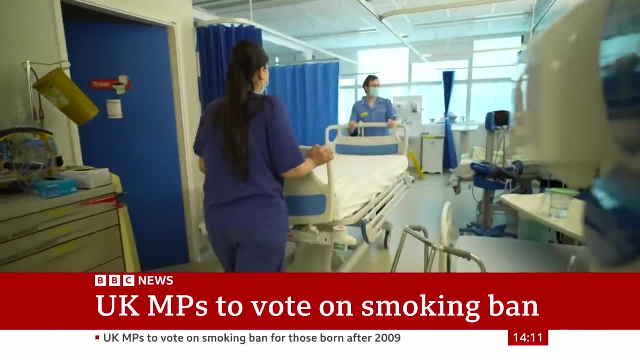 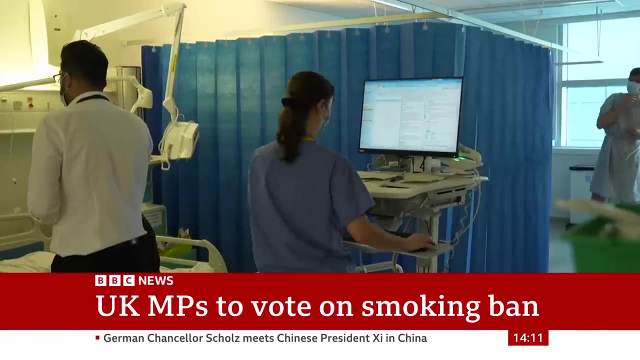 But what I've gone through the last three years I wouldn't like anybody to go through And if I could go back I wish I never started. The harm done by smoking is well-known While documented. it causes lung and heart disease, cancers, stillbirths, dementia and asthma. 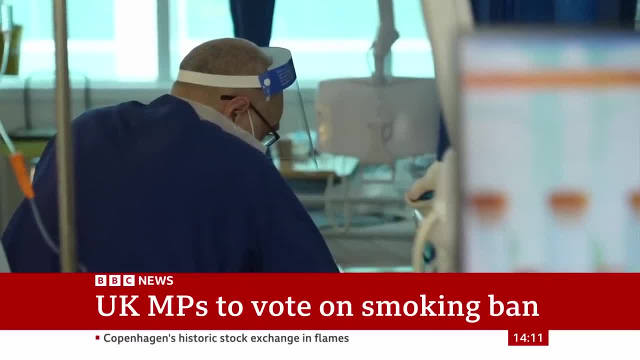 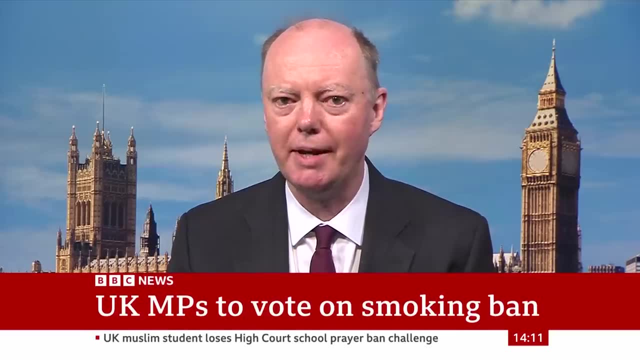 England's chief medical officer, Sir Chris Whitty, supports the ban. People are trapped in smoking at a very young age And once they become addicted, their choice is taken away. So if you're in favour of choice, you should be against something which takes away people's choices. 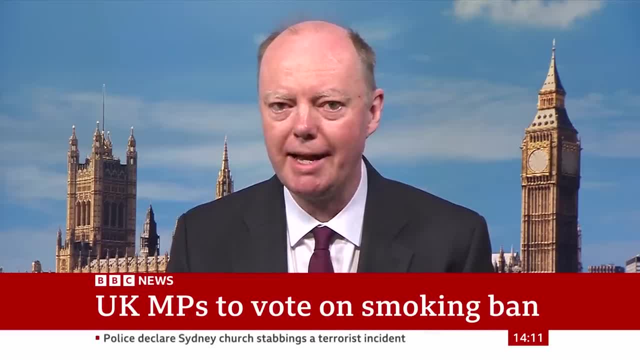 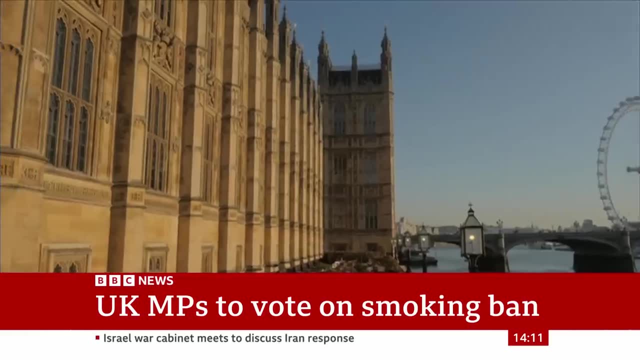 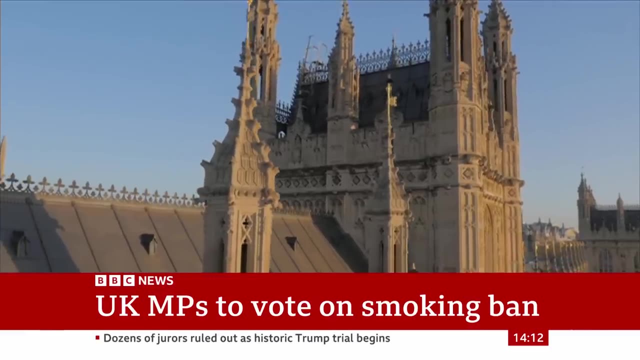 The great majority of smokers wish they'd never started, but now they're in trouble. The Tobacco and Vape Bill, The bill set before Parliament today, represents a huge step change. It proposes that anyone turning 15 this year and all younger generations would be banned from buying cigarettes throughout their lives. 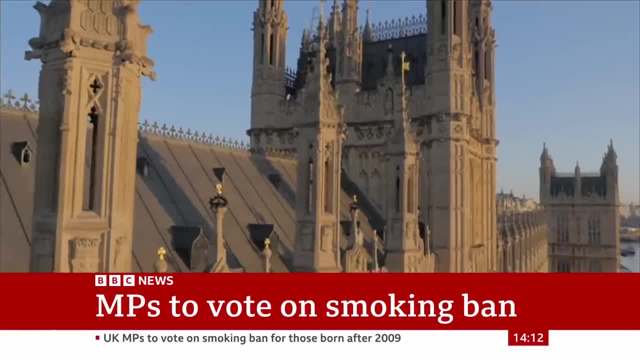 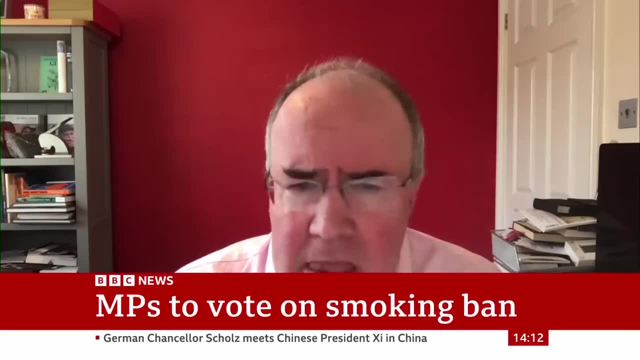 But it sparked a fierce debate about freedoms. What this policy does? it infantilises future adults, Because when you are 18 in this country, you are legally an adult And as such, you should be treated like one. Now look at 18, you can drive a car. 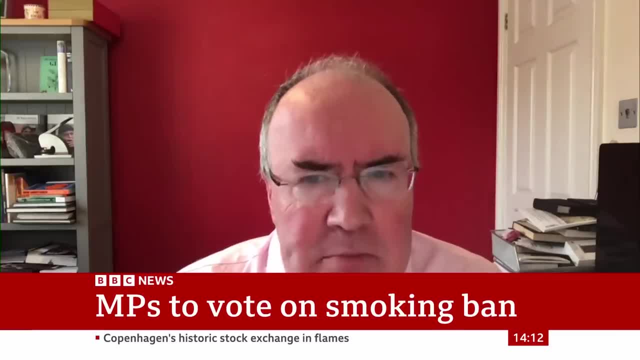 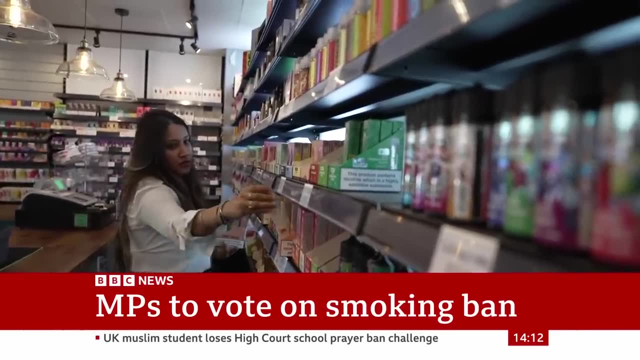 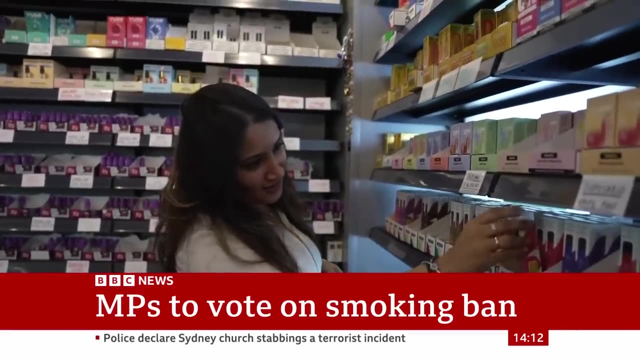 You can join the army, you can possess a credit card, you can buy alcohol And, most importantly, you can vote. The bill also includes new restrictions to tackle concerns about the sharp rise in children using vapes. It would ensure flavours and packaging were less appealing to children, but some are doubtful it will work. 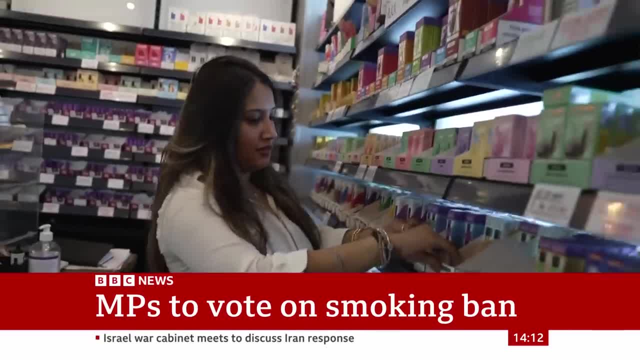 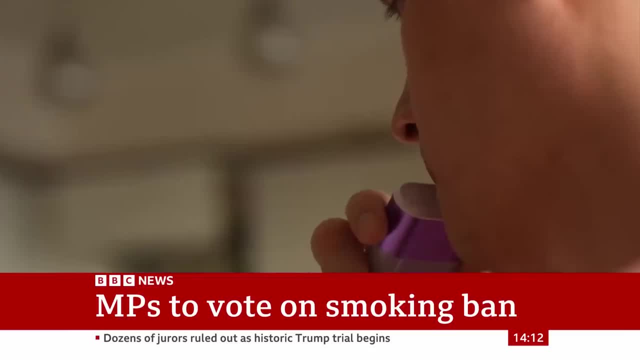 I don't think anybody necessarily looks at the packaging and really, oh, let's just try that. It's more that. oh, it's vaping. it's a cool thing to do, just as smoking was in the 80s. Kids will be kids, they will try smoking, they'll try vaping. 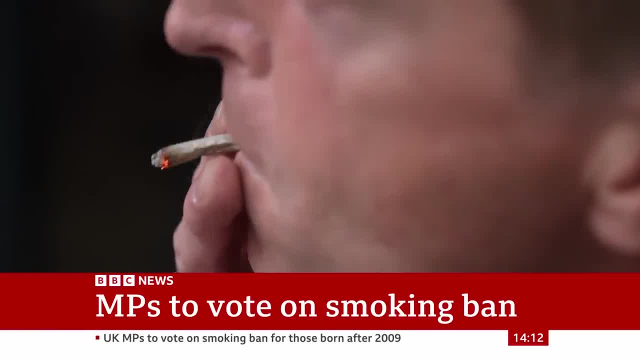 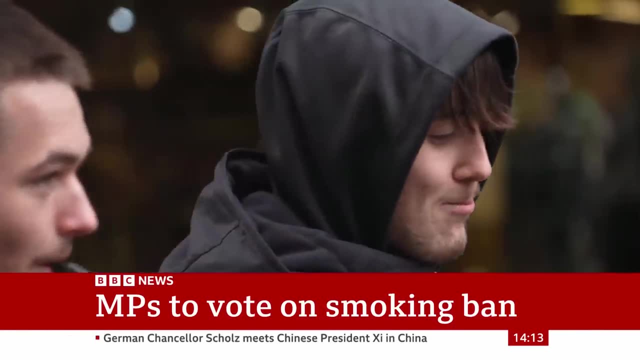 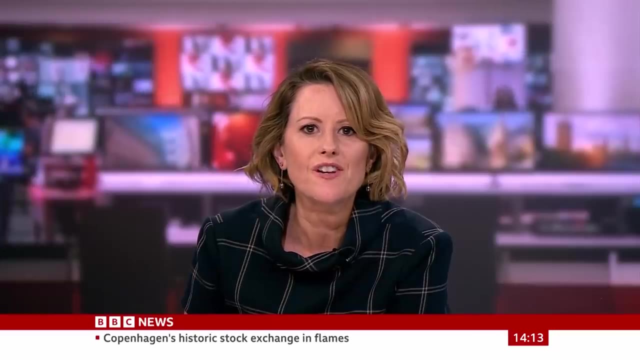 The debate continues in Parliament today, where MPs will be given their first chance to vote on what would be the world's first lifelong smoking ban for younger generations. Sophie Hutchinson, BBC News. While that debate is continuing In the Commons, and Health Secretary Victoria Atkins. has been explaining why she wants the law to be changed. We are trying to move away from this idea that that teenagers- current youngsters- will be able to buy their cigarettes legally in shops from the age of 18 in 2027, precisely because we want to ensure that they can lead longer, healthier lives. Victoria Atkins, the Health Secretary.